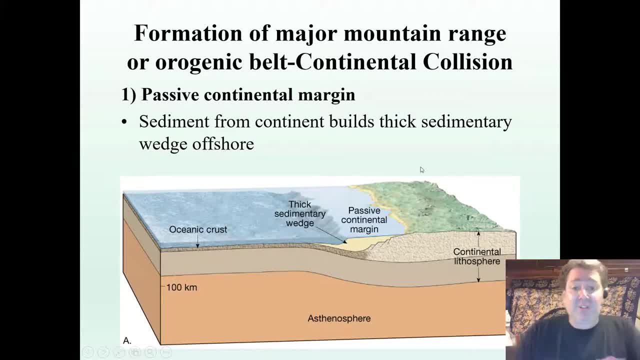 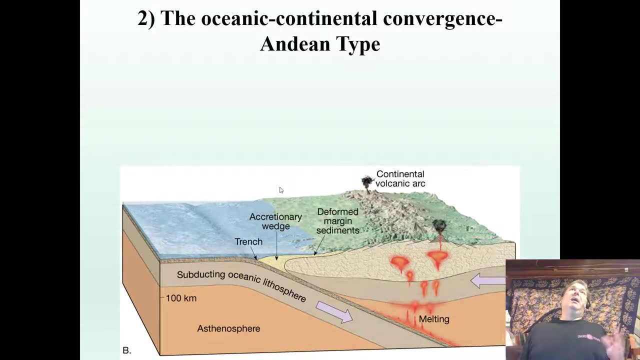 sediment in and deposit it in the ocean right. It creates this very thick continental margin or sedimentary wedge that we call a continental shelf right. But now let's say that plate dynamics change right. So suddenly our Atlantic seaboard becomes an active margin. right There's tectonics going. 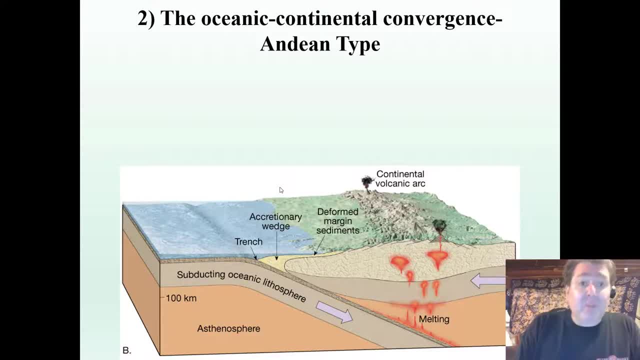 on right there There's subduction stuff like that, right. So we take that nice continental margin right As the plates start to converge, right. A lot of the motion of this collision is absorbed by the process of subduction, right. But not everything gets subducted right. The 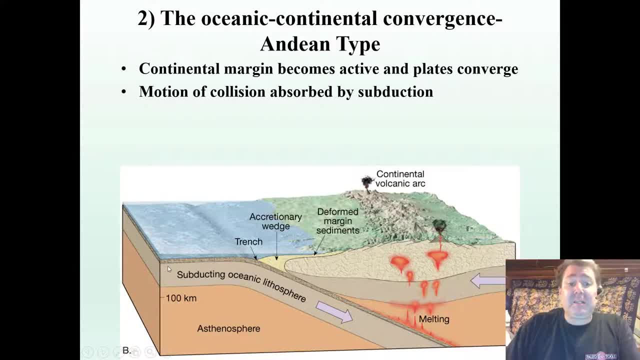 sediments and stuff that have been accumulating on the seafloor right And stuff are going to get scraped up and kind of pushed to the side, you know, onto the side of the continent here right. Subduction of course triggers partial melting. volcanic arc forms back there, We know. 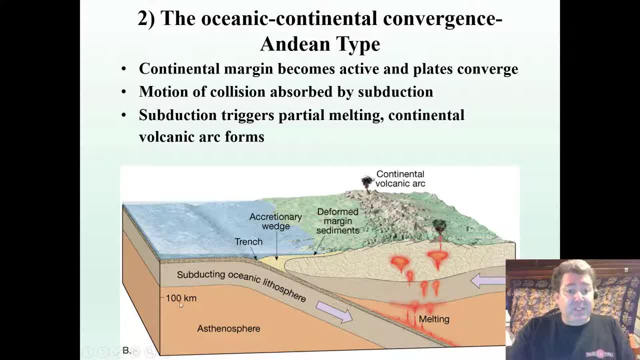 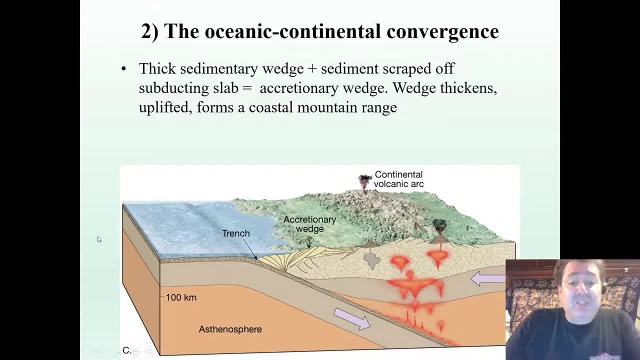 that already right, But let's follow this area as it evolves through this active margin, right? So as you see here now, all those sediments and stuff getting squished together. as you imagine, there's a lot of compression happening in there. It's pushing a bunch of these sediments together. 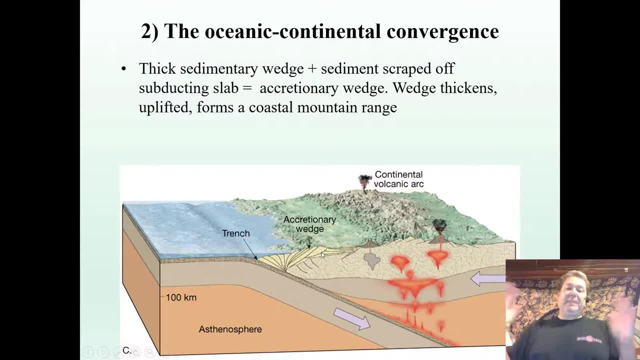 and shoving them together. And because we have a space tissue there, right, Not enough space, we're pushing together, we're shortening, we're thickening, We've got a bunch of reverse faults in there squishing things together. You can see. 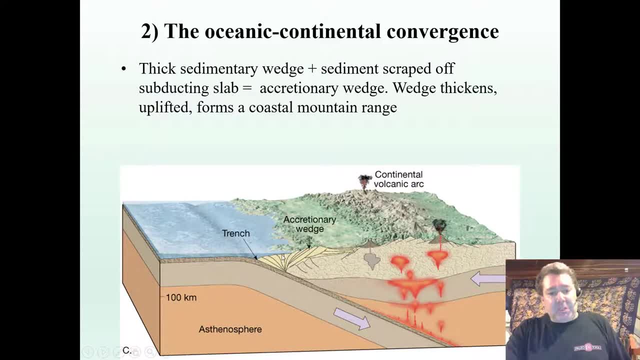 all those right here, right, And that basically you know, eventually we'll squish together and lift up enough where it creates, you know, a kind of a coastal mountain range, not a volcanic mountain range, right, An aseismic or non-volcanic mountain range. just basically made up this. 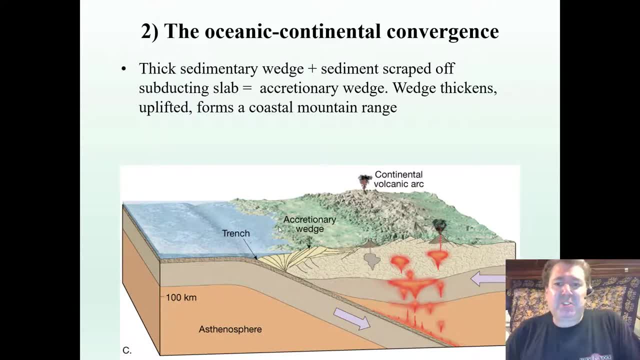 smashed up, messed up, beat up, stuff that's been scraped to the side of the continent, right? So what we're going to do is we're going to take a little bit of this. we're going to take a little bit of. what you end up with at the end are two essentially parallel zones of mountains, right? 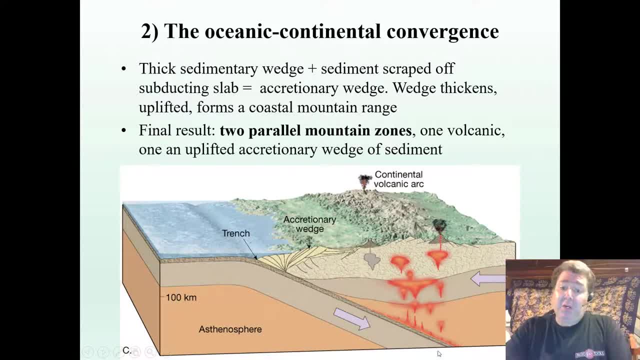 The one inland being a volcanic set of mountains, showing where you get down to that point where water's being driven off the plate and causing partial melting right, And the other one that uplifted and smashed up a cretinary wedge which used to be our continental margin right. 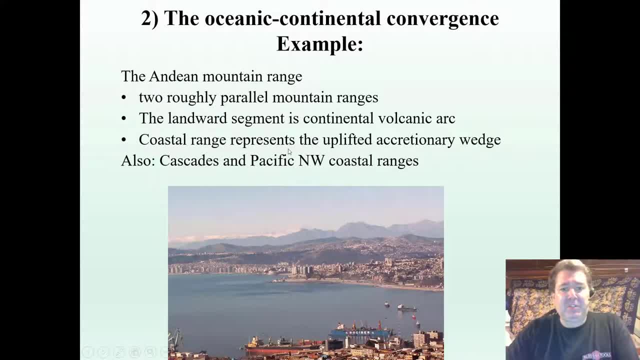 You can see this in the Andes. You can also see it in the Cascades in the Pacific Northwest right. So you have this, this back farther. Those are the, the volcanic mountains. These in the front here are the, the non-volcanic uplifted sediments, and 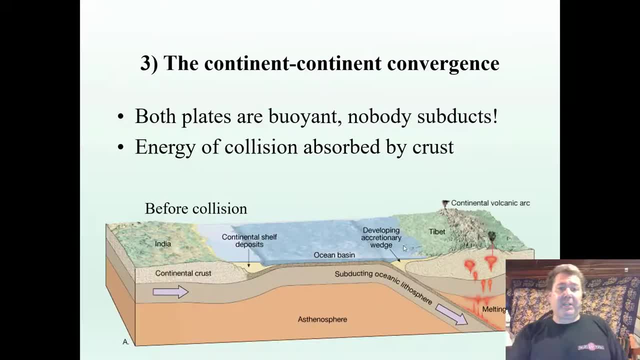 crapped mountains, right? So you end up with two kind of parallel change, right? So let's look at continents: continent style convergence, mountain building, right? So in this case you know, both the continental plates are buoyant, so nobody gets subduct, right? So instead of that collision, 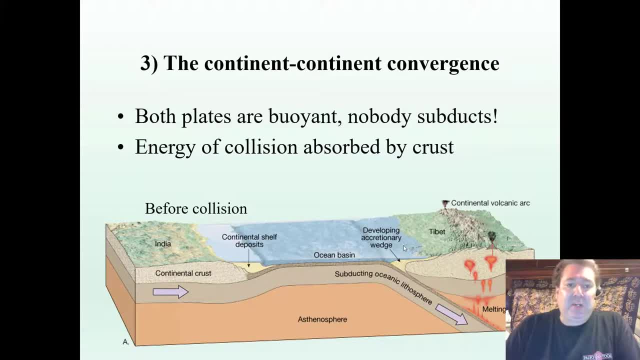 you know, a lot of it going down the trench with the, with the subducting lithosphere, right, It gets absorbed by the crust So you end up with two kind of parallel change right. So it's like two cars playing chicken and nobody backs off, right, And always kind of our, you know. 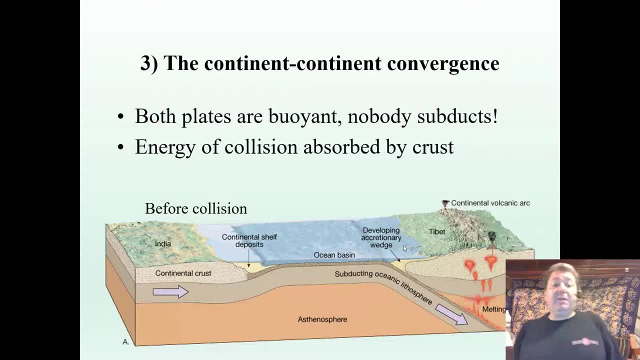 primo example of this is the Himalayan mountains. right, So about 40 million years ago, this little subcontinent of India smashed into Asia and started to develop the Himalayan mountains. Why? Because there we have, you know, again a space issue. not enough space, things have to shorten and thicken. 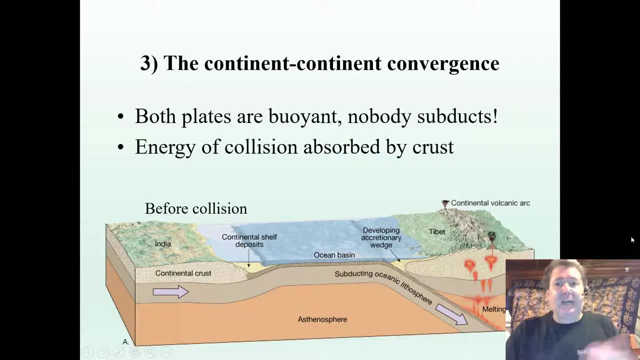 creating mountains: right, But it wasn't always a continental, continental convergence. right Before these two land masses met, what you had was your standard right Continental oceanic subduction zone. right, With India just kind of riding along for the ride. right Once India hits this continent right, That's when 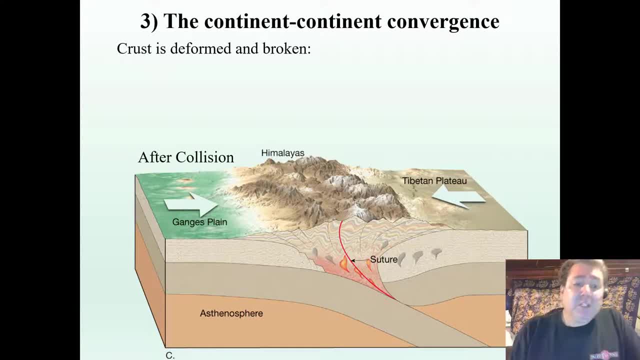 we're going to change plate dynamics, right. So here's before, right, And it's moving along, and he's just cruising along and here's when it hits right. So this is after the collision, right. So we have the the Ganges. 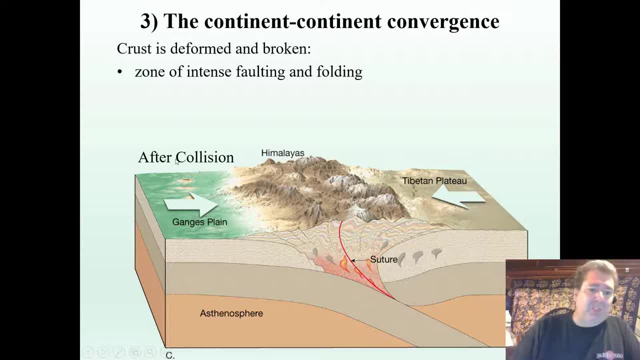 plane here in India, right, We also have the Tibetan plateau, So this is originally India, This is originally Asia, right. And of course, as you imagine, this zone in here is just intense with faulting, folding right. What kind of faulting? Reverse faulting, because that's what shortens and 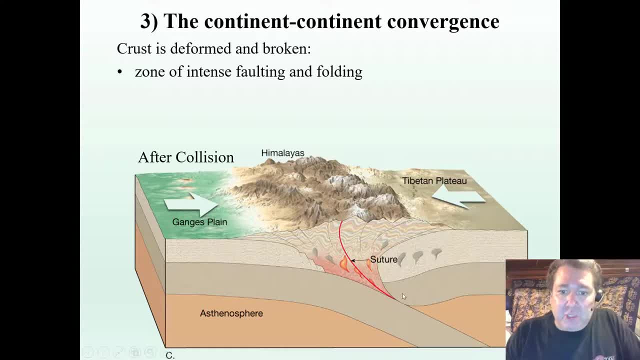 thickens stuff, right. And also you'd notice that there's this suture here. There's a specific type of rock called, I believe it's, mylonite. that can tell you where that original smashing of the two continents, everything on this side is originally a um uh, India, and everything on this side is